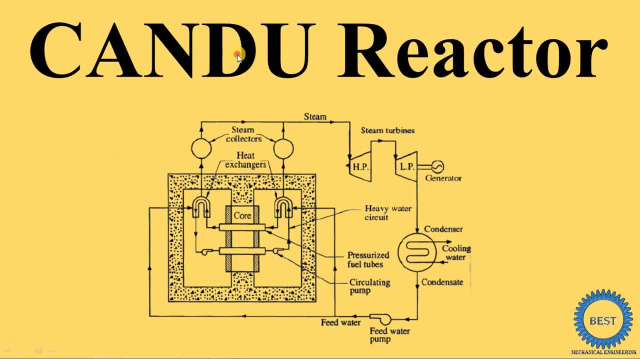 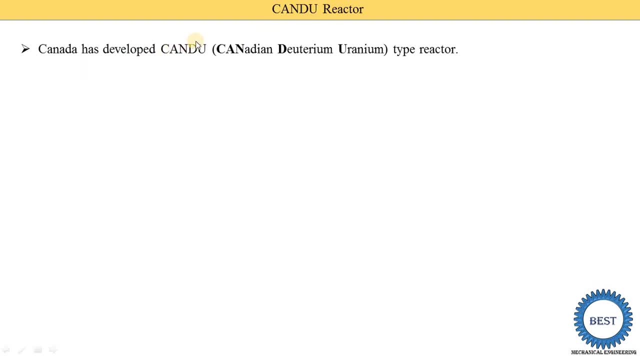 In this video I explained CANDU reactor. First we understand what is the meaning of CANDU. Canada has developed CANDU type reactors. CANDU means first, three digit is indicate Canadians. Four digit is D, D is indicate deuteriums and the U is indicate the uraniums. 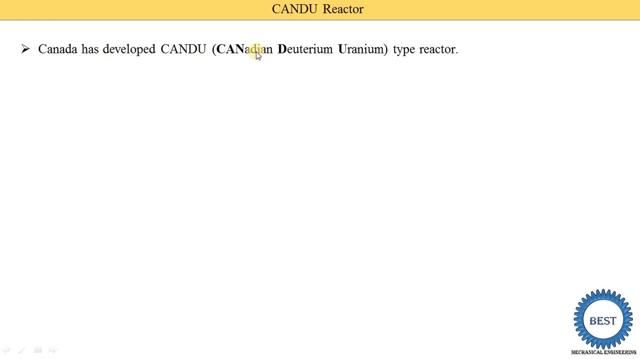 Okay, so it is developed by the Canada. That's why its name is given as the Canadian deuterium and uraniums. So deuterium is used as a moderators and this uranium is used as a fuels. Okay, so these names are combination of the three terms. First term is indicate the development. 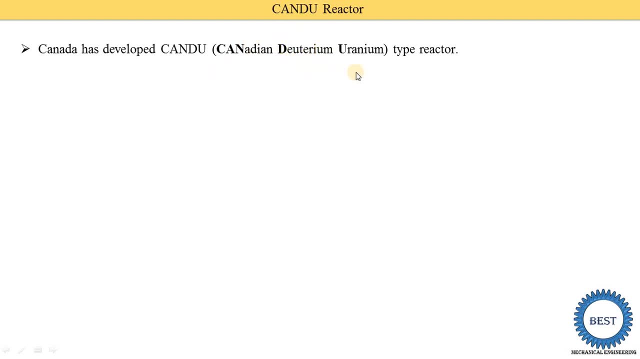 of country. Second one is used as the moderators and the third one is indicate the fuel used in a reactors. It use pressurized heavy water. PHW means deuterium, So it is used in the deuterium oxides. Deuterium oxide is also written as the d2o as a moderators. Okay, so these deuterium oxide is used as a moderators, as 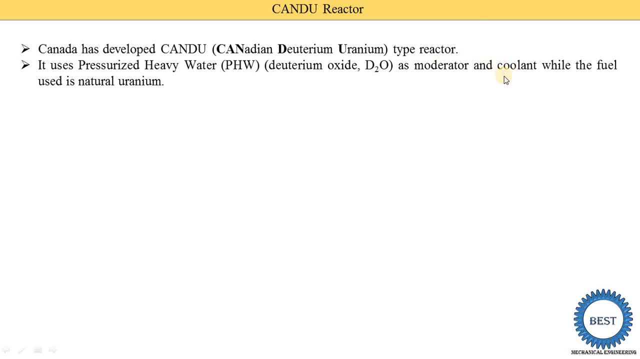 Well as the coolant means. moderator and coolant material are same, Why the fuel uses natural uraniums. So fuel is uses natural uraniums. These reactor are more economical To those nations which do not produce and rich uranium, as the enrichment of the uranium is very costly. Okay means it is the benefit for the country which are not able. 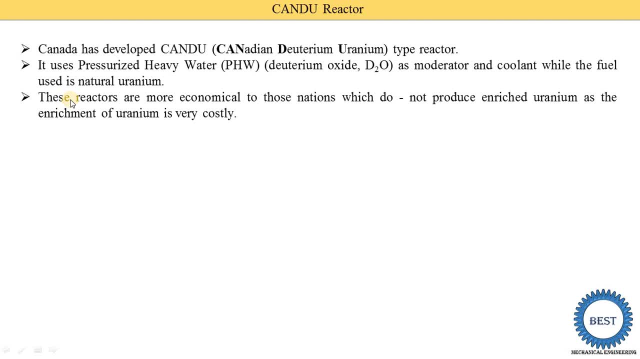 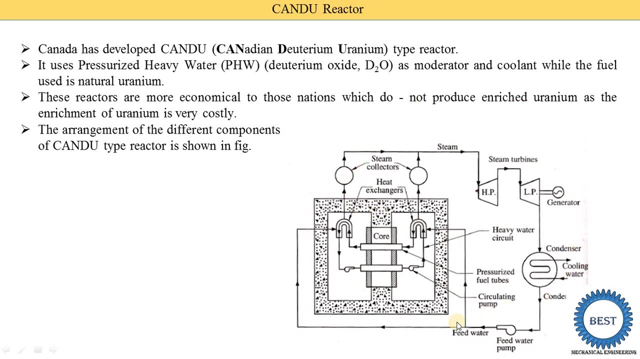 To create enriched uraniums. Okay, so they can use the natural uranium as a fuels in a can do reactors. The arrangement of the different components of the can do type reactor is shown here In these figures. okay, so here you see. these are the diagrams of the can do reactors. 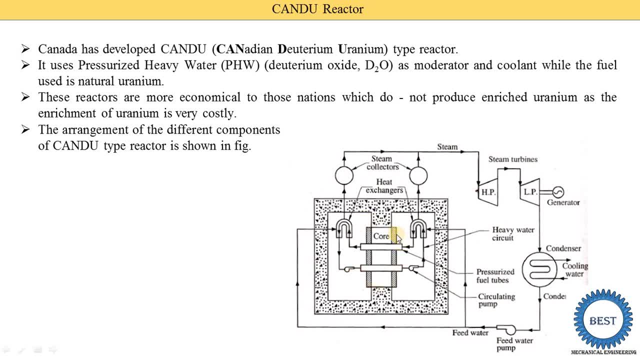 Okay, so suppose we starting from this center parts, So it is the core. Okay, in a core. you see, this is the Pressurized fuel tubes. are there? Okay? So this is the one pressurized fuel tubes. This is the second pressurized fuel tubes. in this pressurized fuel tubes The fuels are put it Okay. 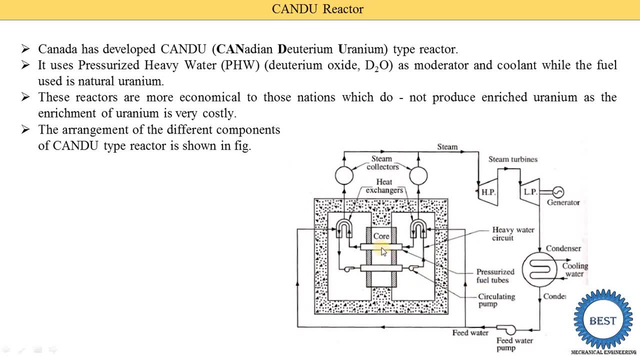 That's why its name is given: pressurized fuel tubes. in a pressurized fuel tubes, That is, a number of bundles are there and In this bundles there is a Number of pallets are provided that we discussed later on. Okay, so this pressurized fuel tube is 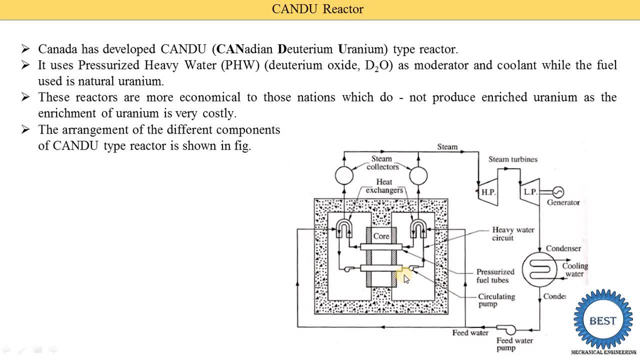 create the heat energy due to the fission of the uranium materials. okay, and this heat energy is carried by this Heavy water. circulating in this pipe means here, you see, heavy water is supplied in this core. They absorb the heat energy and this transfer heat energy to the heat exchangers. Okay, so in these heat exchangers, 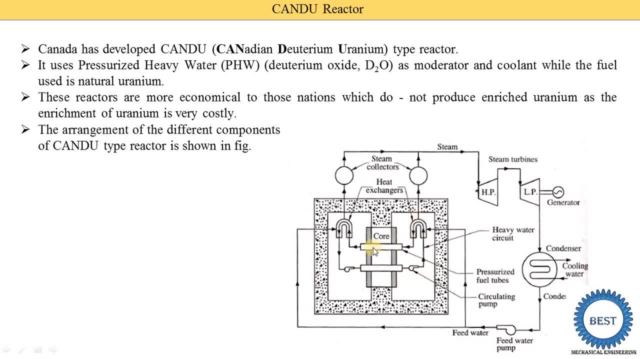 Here this heavy water is circulating, means d2a is circulating. This, the d2o, is supplied heat energy to the water that is passed from these other pipes in these heat exchangers. okay, and again this Heavy water is coming and it is again passed from these pressurized fuel tubes. So this 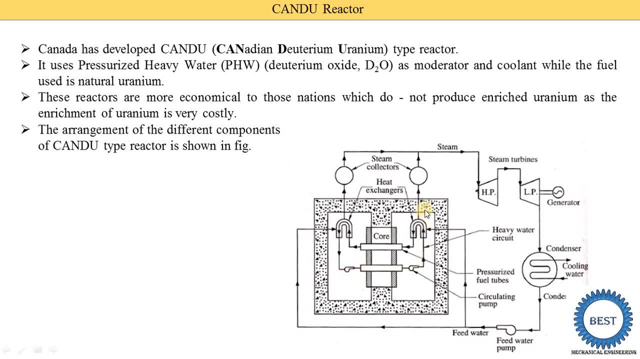 Heavy water is again absorbed, the heat energy, and then it is supplied to this second heat exchangers. So here they are. also Supply heat energy to the water and the water is converted into the steams. Okay, so this is the basic functions of this pressurized tubes. okay, and this is the steam collector. so here. 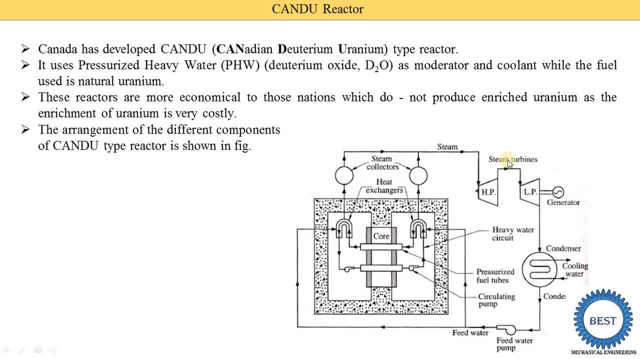 steam is collected, then the steam is supplied in high pressure turbine, then it is supplied in low pressure turbine, then condensers and feed water pump, and again feed water pump is supplied in these heat exchangers. okay, so in this heat exchanger- here you see from the one sides. 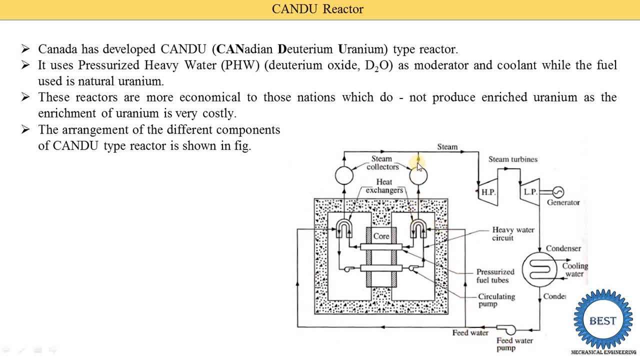 this feed water is supplied and this feed water is converted into the steam and from the pipe heavy water is supplied. so heavy water supplied, heat energy to this feed waters. and feed water is converted into steam and the steam is supplied to this turbine. so in this reactor the fuel is. 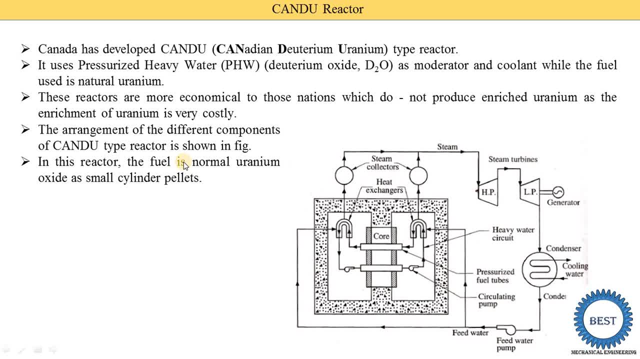 normal uranium oxide as a small cylinder pellets. okay, means the uranium fuel is converted into the small cylinder pellets. now what is the size of the cylinder pellets? so the pellet are packed in a corrosion resistant zirconium alloy tubes and its size is nearly 0.5 centimeter. long means its length is 0.5. 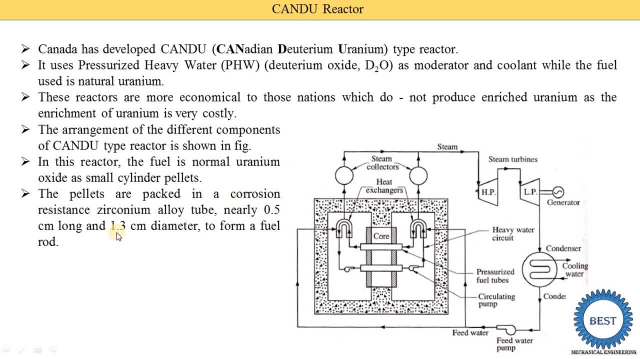 centimeters and 1.3 centimeter diameters to form a fuel rods. okay, so what is the size of fuel rod? that is a 0.5 centimeter long and 1.3 centimeters diameter. the relatively short rods are combined in a bundle of 37 rods. okay, so when we 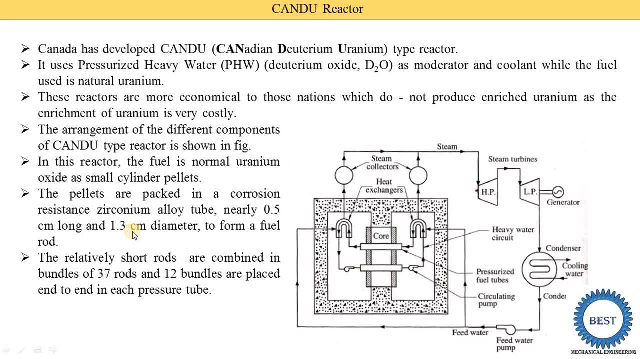 combine the 37 rods. okay, so it is called as the one bundles and that is, our 12 bundles are place end to end in a each pressurized tubes. okay means here you see this diagram: 2 pressurized tube is there in a 1 pressurized tube there is a. 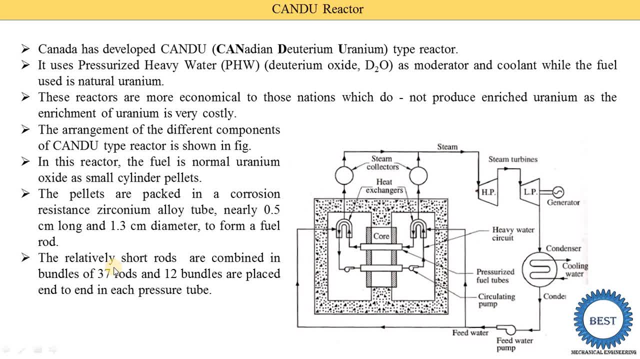 12 bundles are there. in a 12 bundle 37 rods are there. okay, so total, how many rods are there in a one pressurized fuel tube? that is a 37 into Não dois size of this one fuel rod is the 0.7 centimeter long and 1.3 centimeters diameter. the total mass. 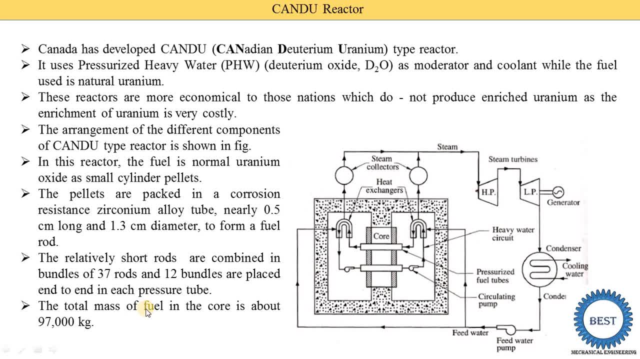 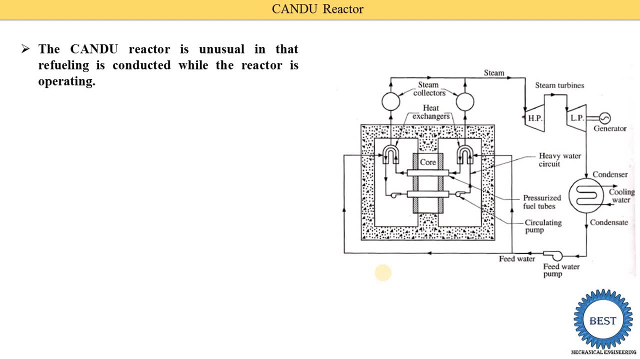 of fuel in the core is about 97,000 kilojoules. okay, so that is the number of fuel tubes are there. okay, so total weight of the fuel is 97,000. so in a kendo reactors we are able to refuel the core in a operating condition. means we not need to stop the reactor for the refueling of a. 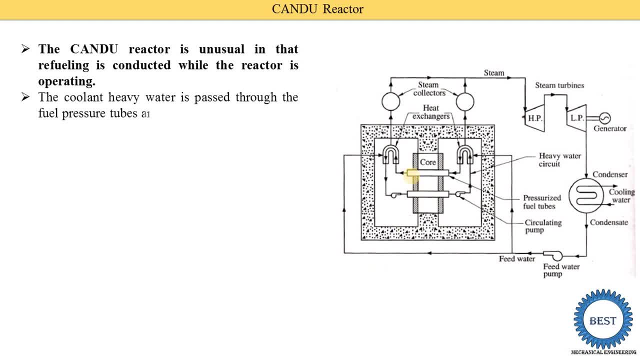 fuel, the coolant, heavy water is passed through the fuel pressure tubes and then operating heat exchangers. okay, so here you see. these heavy waters are continuously recirculated in these circuits. okay, and this heavy water is passed from the core and in the core they absorb the heat energy and 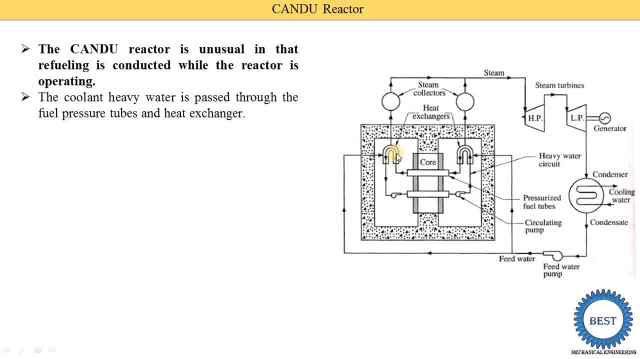 this absorb heat. energy is supplied to the water against the recruiter and then the� a heat exchanger. so in a heat exchanger that is a, two mediums are there. one medium is the heavy water and the second medium is the feed waters. okay, so this heavy water is supplied heat energy. 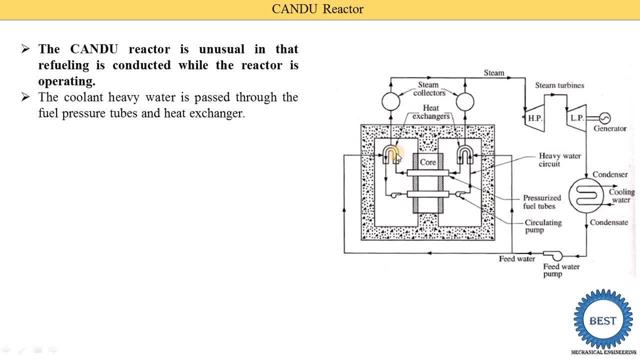 to the feed waters, and feed water is converted into the steam. the heavy water is circulated in the primary circuit in the same way as with the pwr, and the steam is rise in the secondary circuits and transferring the heat in the heat exchangers to the ordinary waters. okay, so this part is called. 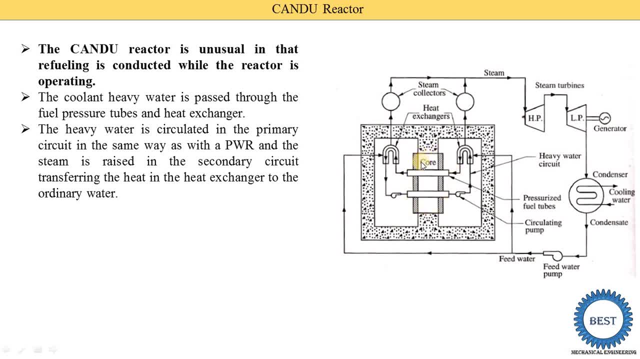 as the primary circuits. okay, so in a primary circuit. these cords are there in a core, pressurized fuel tubes are dead, circulating pumps are there and these heat exchangers are considered in this primary circuit and this part is called as the secondary circuits. okay, so in this. 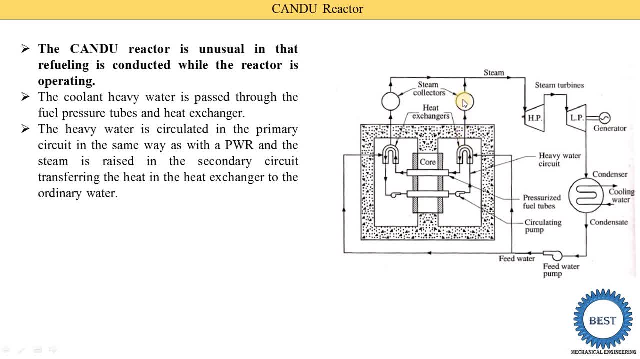 heat exchanger, the steam is produced, and this steam is supplied in the steam collectors and then, after it is supplied into this high pressure turbine, then after it is supplied in the low pressure turbine, so in it, this turbine, this mechanical work is produced, this mechanical work is supplied to generators, and generator is produced, the electricity. 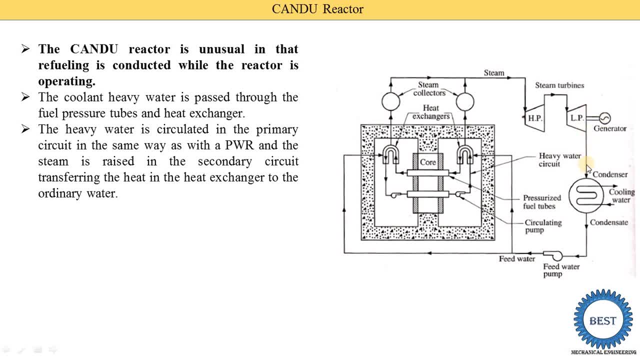 then, after steam coming out from the low pressure turbine is supplied to this condensers, in the condenser it is condensed, means the steam is convert into the water and this feed water is again supply to this heat exchangers. okay, so this way this cycle is. 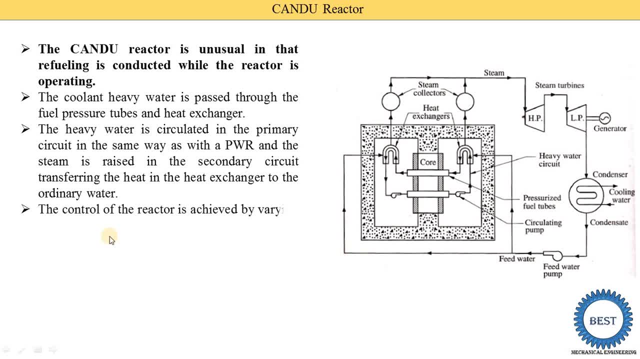 continuously run. the control of the reactor is achieved by changing the level of moderator in the reactors. okay, so, as a moderator, we use the d2o. okay, so if we change the level of the moderators in these reactors means changing the level of the moderator, means changing the level. 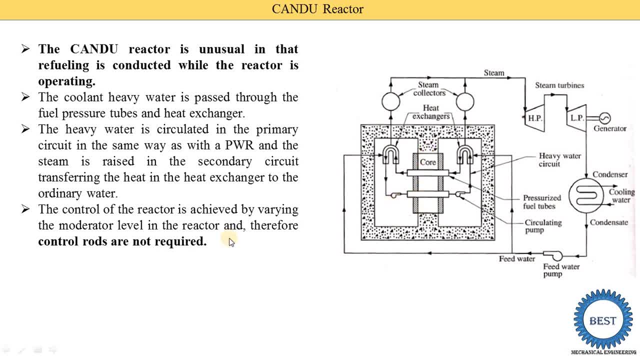 of d2o in this code, then what happen? we are able to control the reactions in the reactors. therefore the control road are not required. so in a can do reactors, control road are not used. cadmium roads are used to start and shut down the reactors. okay, so in earlier cases, what we 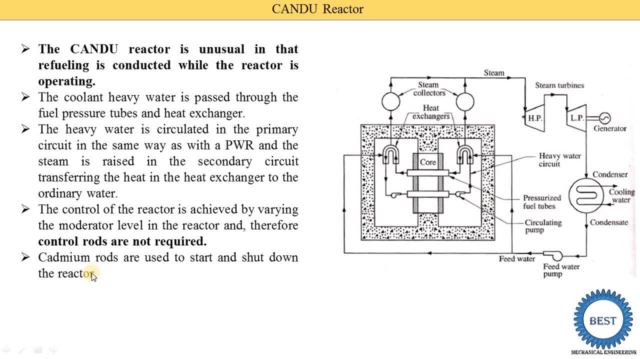 study the control road are used to start the fission reaction, control the fission reaction and stop the fission reactions. okay, but in this can do reactors, we are not use the control road. okay, so by changing the level of moderators we are control the reaction, but how we start and 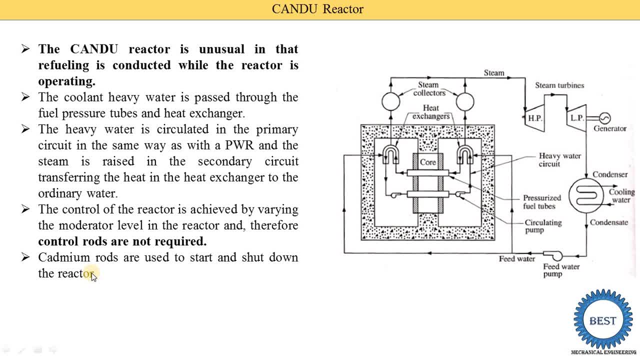 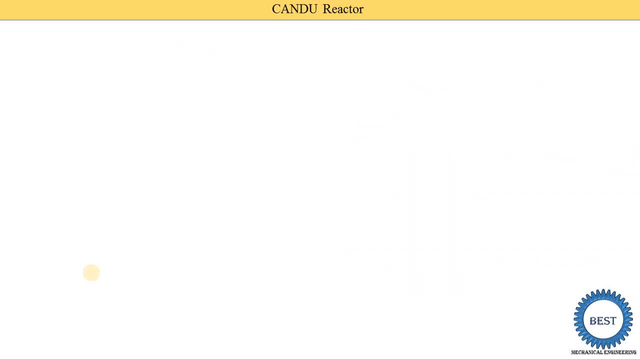 stop the chain reactions. so for starting and stopping of the chain reactions we need to use the cadmium roads in a can do reactors before moving towards the advantages and disadvantages of the can do reactors. i request to like the video and subscribe my channels for watching the more video related to nuclear power plants or power plant engineering subjects or